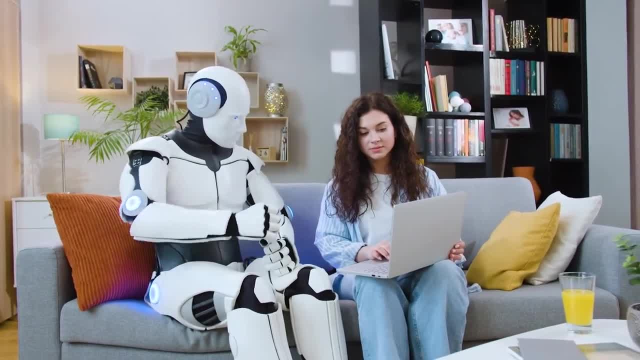 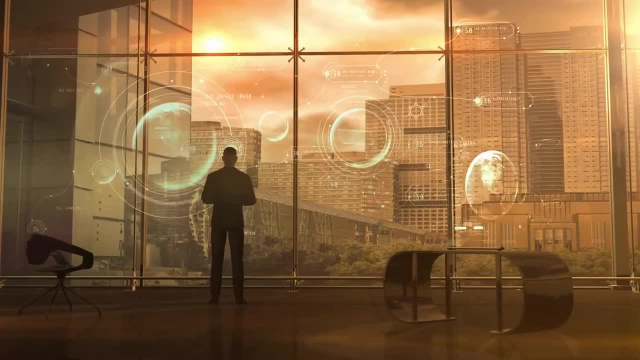 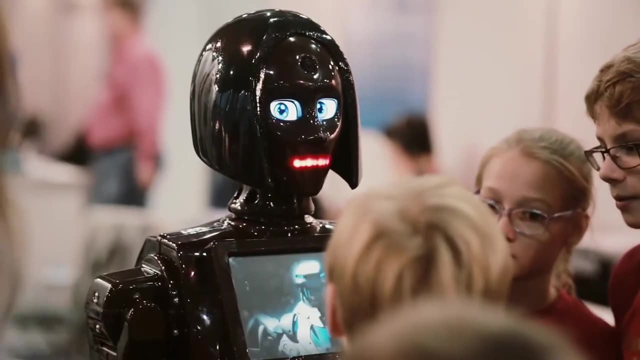 the digital supply chain improves and more and more smart devices are made. Also, telecom companies will work harder and smarter to keep up with the fast-paced and complicated global economy. They will have to figure out how to get along in a world where customers are picky and want new updates all the time to make communication easier than ever. 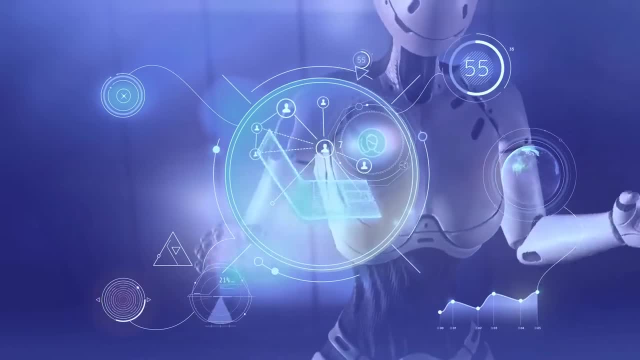 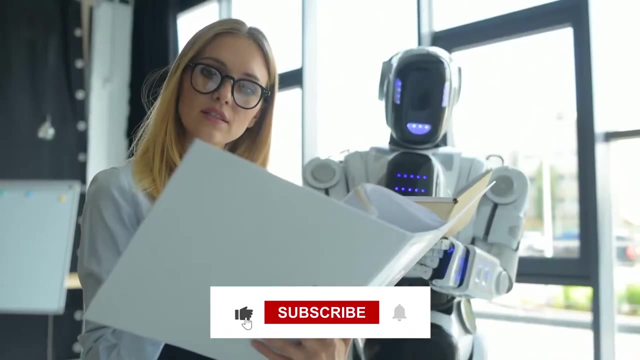 In today's video, we will discuss the future of telecommunication technology. However, before we begin our video, we would greatly appreciate it if you would subscribe to our YouTube channel and also press the bell icon. Let's get started. Industry Restructuring. 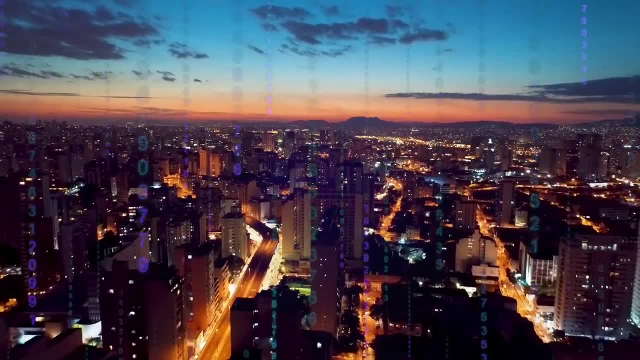 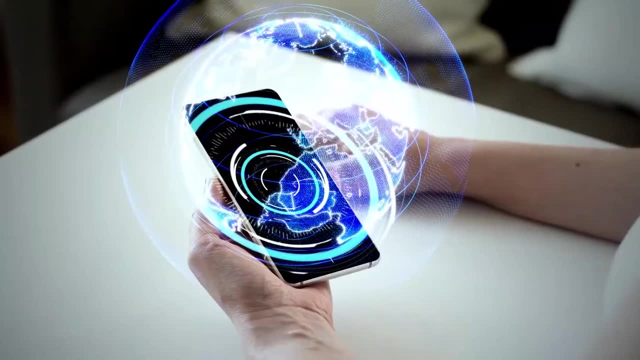 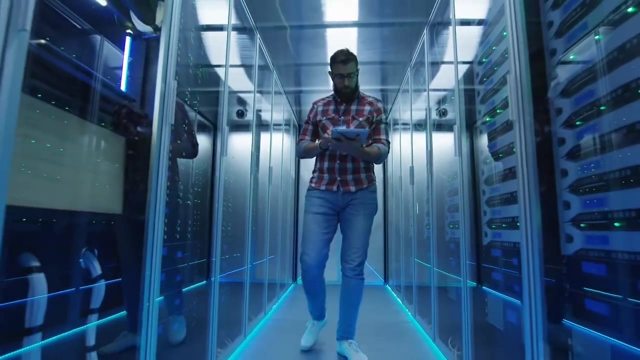 To get the support and trust of customers again, there needs to be a dual transformation and a restructuring of the industry. To stop the network from becoming a commodity, the telecom industry will have to change the way it does business at its core. They will have to come up with a solution that works for everyone To get the most out of the 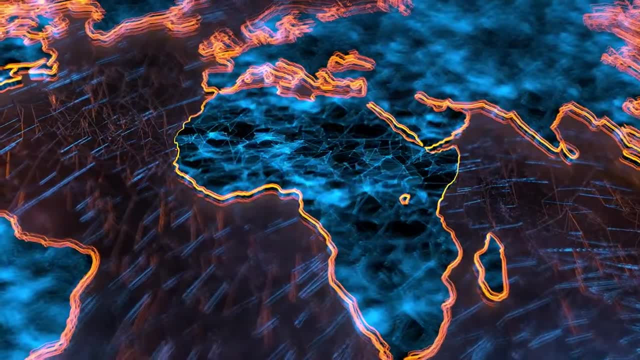 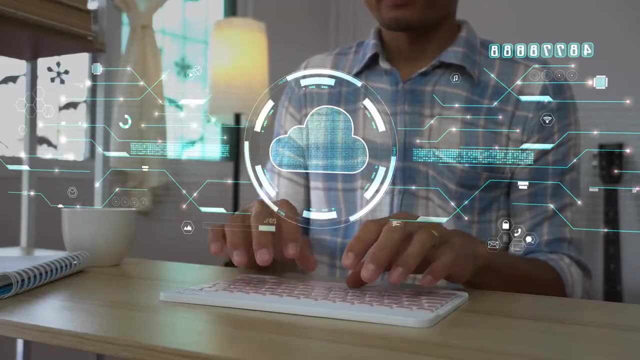 changes to the network, they will have to understand why they are being made To make the system more resilient and secure. networks need to be customized and made more secure. At the same time, they have to reduce latency, jitter, interference and the number of errors. 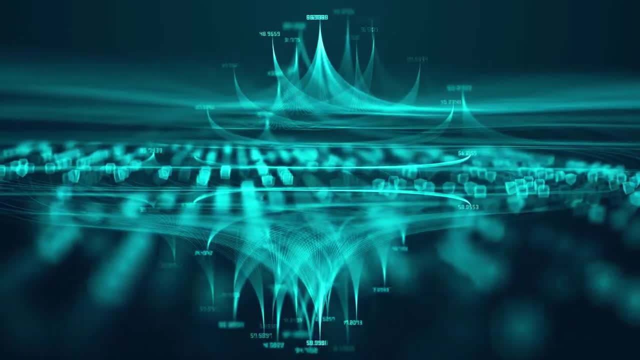 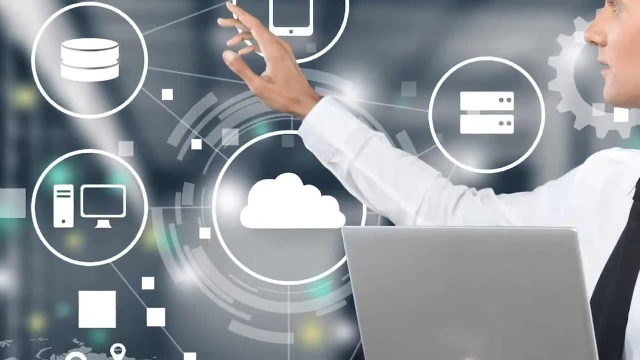 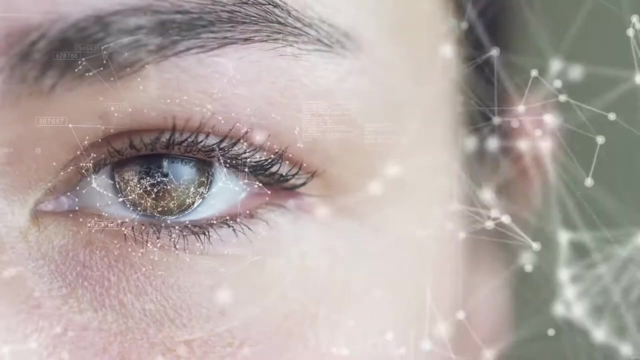 In order to offer trust network services, some changes must be made. There should be four parts to the trust factor. There are four of these: Privacy and security, trust control and support for engagement For privacy and safety. the telecom industry should focus on identity management and cryptography techniques. 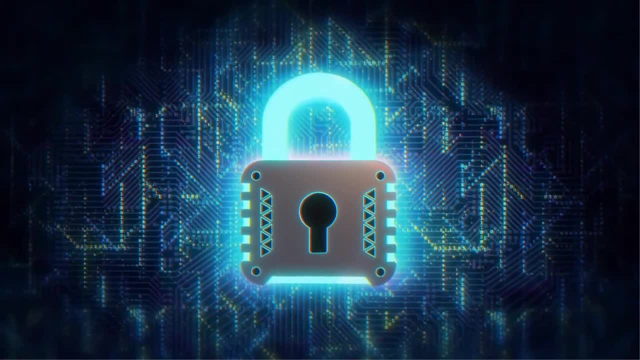 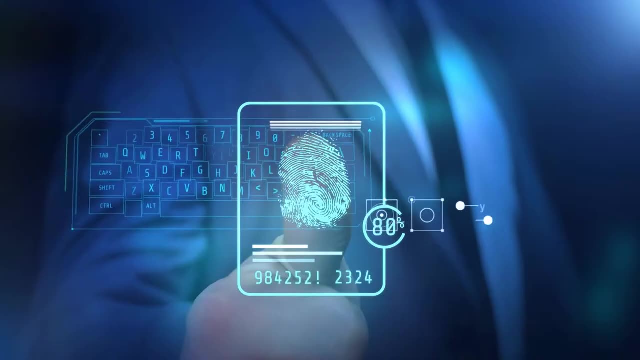 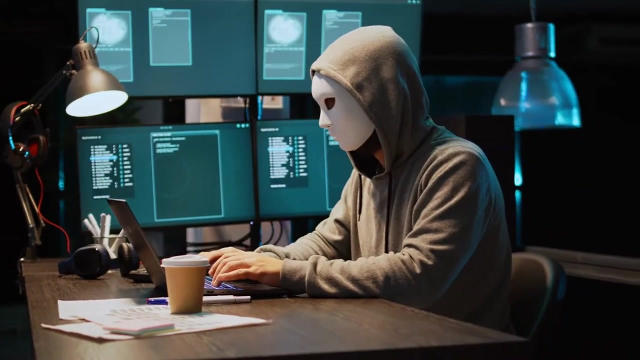 used by the military. These will make sure that transactions are done correctly and that communication and information transfer are at their best For trust. networks will have to focus on attestations and certifications that are known and have been proven. They have to put these into a shared ledger. A trustworthy environment can be made. 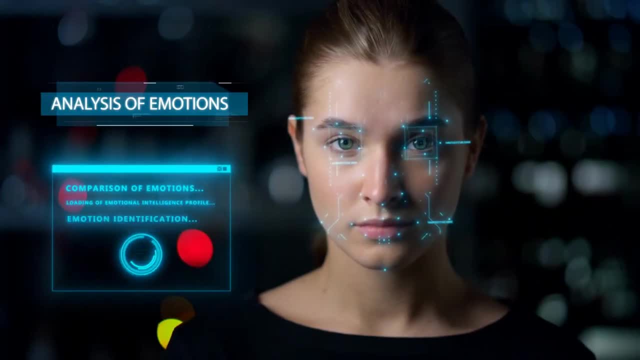 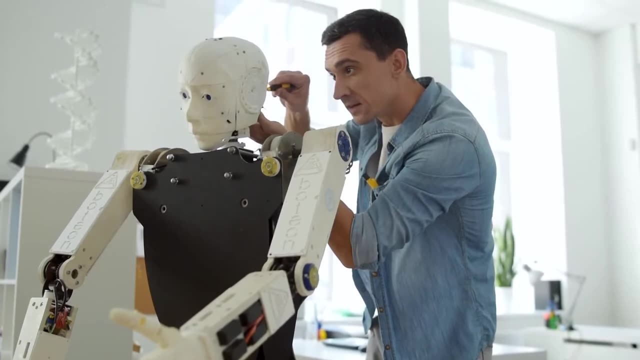 by keeping records that can't be changed or lost. Supporting new and advanced technologies will be a top priority in order to get results that are driven by success, bring down costs and make customers happy. For better control, the telecom industry might focus on self-sovereign. 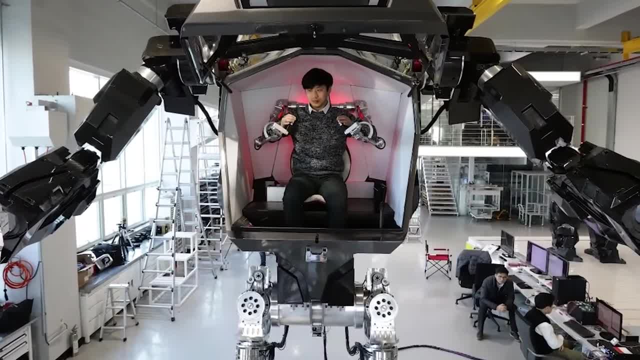 identities that have been verified and on being more open Analytical Maintenance. AI analytics will be very important in the future of investment. A lot of people are focused on AI analytics that doesn't have a many-male thing to do with the system, and I think this is very important. in the future of development and impact in the future as well, because that's where we are. AI analytics will be very important in the future of investment. AI analytics will be very important in the future of investment. AI analytics will be very important in the future of investment. AI analytics will be very 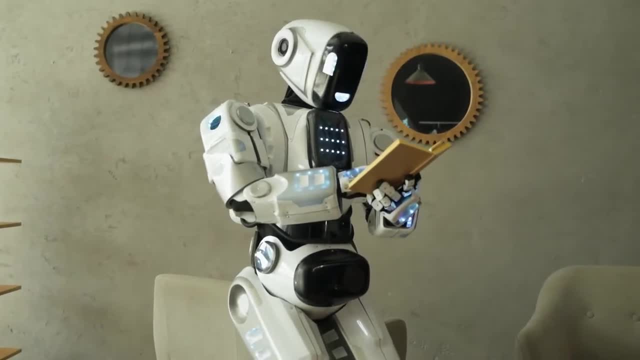 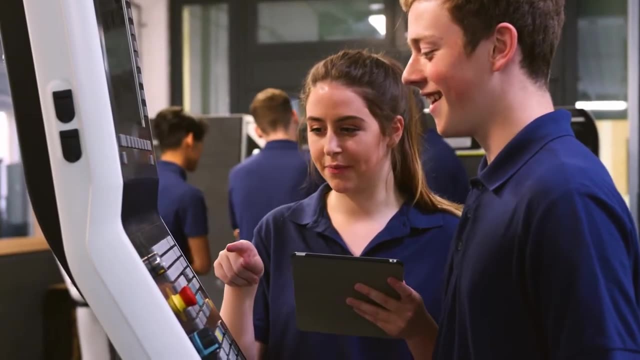 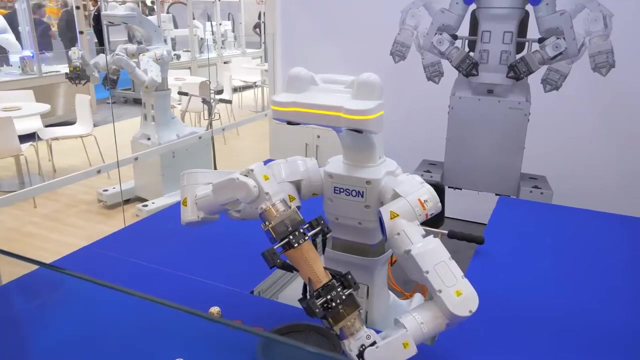 very important in the future of telecommunications. I will be used more in the telecommunications business. It will help top companies offer more advanced services by letting them use machine learning techniques and complex algorithms. All of these will help predict the future based on what has happened in the past. 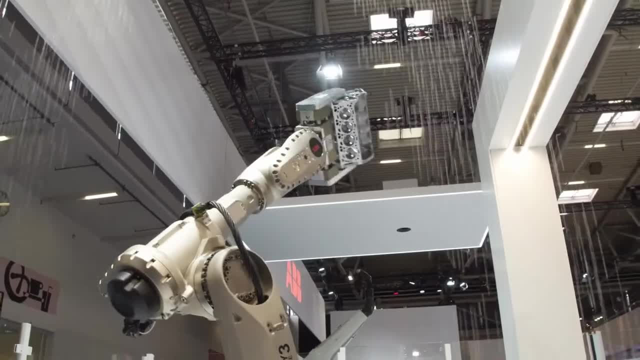 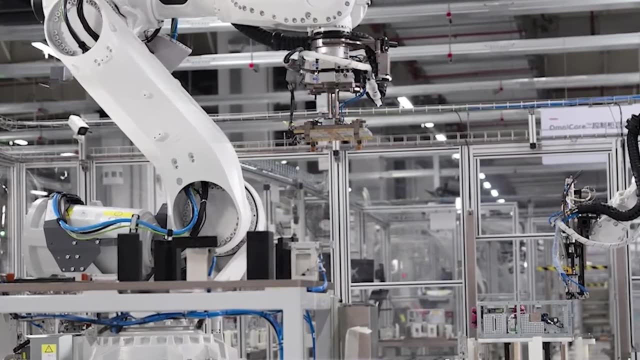 Also, the telecom industry will be more focused on data-driven insights in the future. These insights will keep track of how the equipment is doing and, based on the data patterns, predict when it might break down. Also, it can help get things fixed. 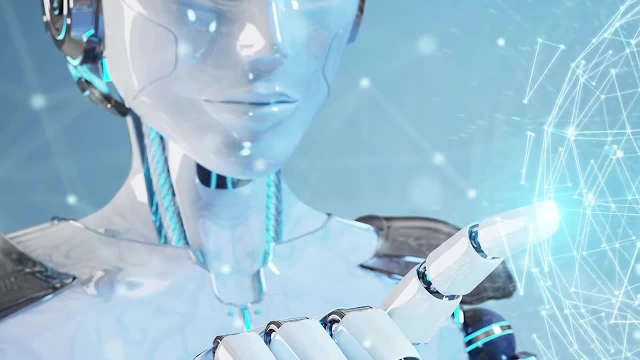 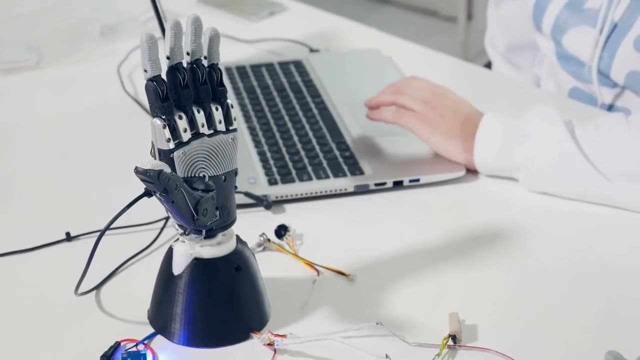 These new technologies could make customers happier by helping them solve their problems faster and better in real time. RPA, which stands for robotic process automation, is a type of technology that will help the telecom industry handle rule-based back office tasks and large amounts of repetitive work. 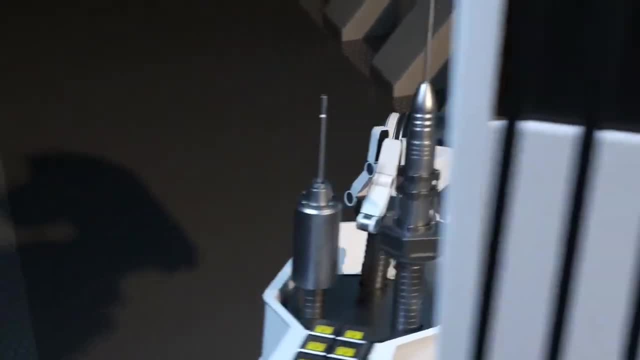 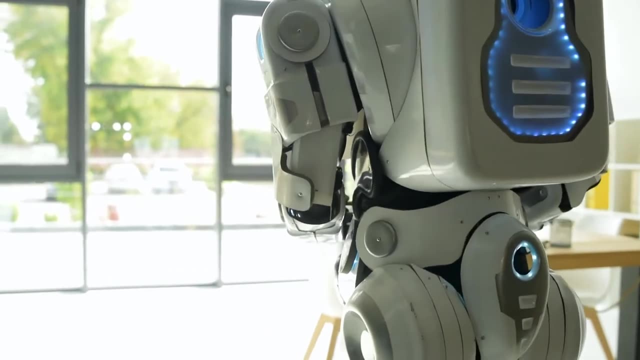 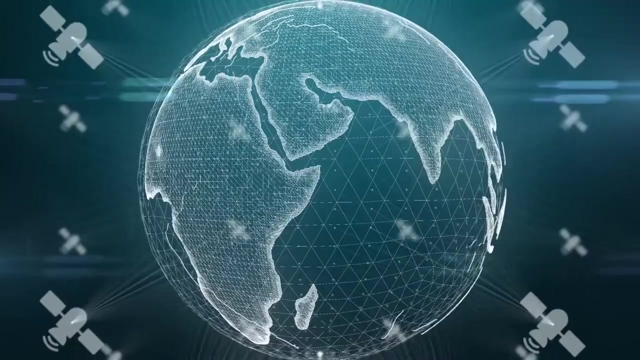 more easily and quickly In the future of telecom. RPA technology will handle tasks that take a lot of time and work. It can make a lot of work easier, like managing employees, entering data, filling orders and billing 5G. it will work with more than just 4G. 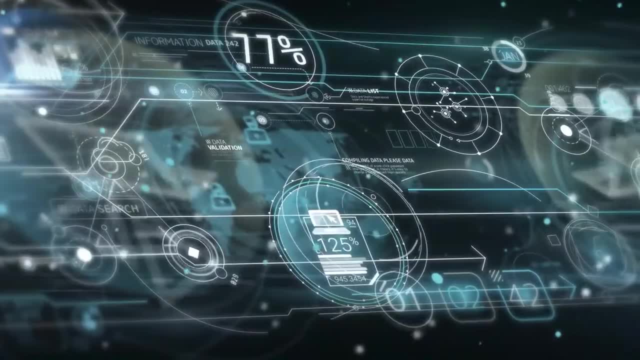 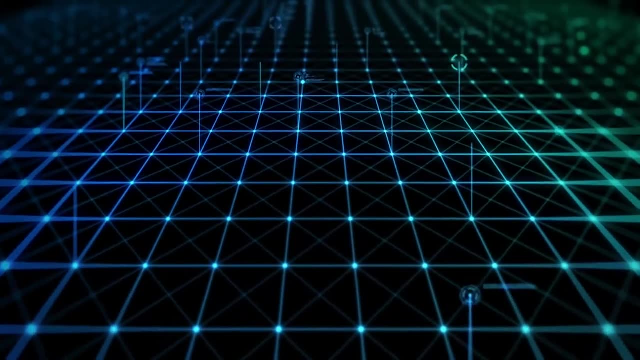 The network providers are working on 5G because they think it is the future of the telecommunications industry. Ford, Google and Uber are just a few of the big companies that are working on 5G and trying to give it a shape in the near future. There is already a first try at 5G. Once it's put in place, customers can expect more speed and efficiency. Mergers in the telecom industry. it's not new for companies to merge or join together, but the industry could be in for a lot more in the future. 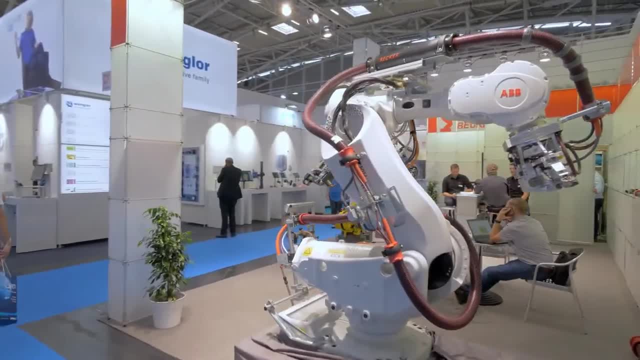 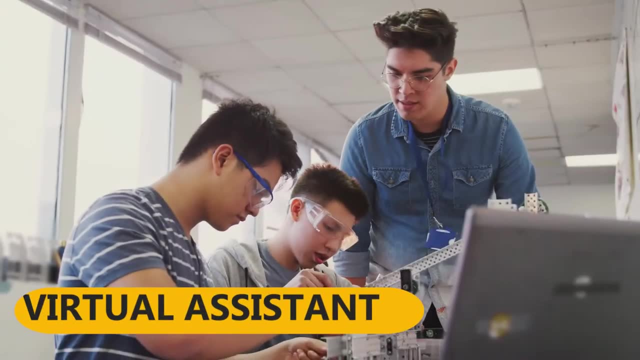 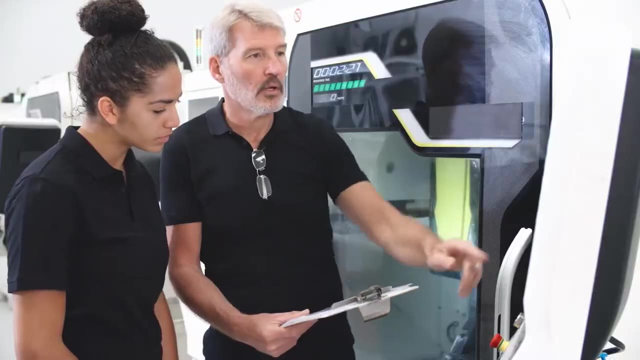 There could be a lot of interest from telecom companies to merge, for the better Customers will get, better service through consolidation It will make new things possible. Virtual assistant- virtual assistants are used a lot by telecom companies to keep track of customers and answer their questions about setup installation. 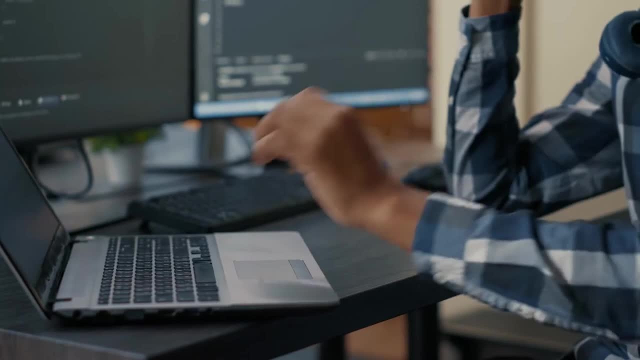 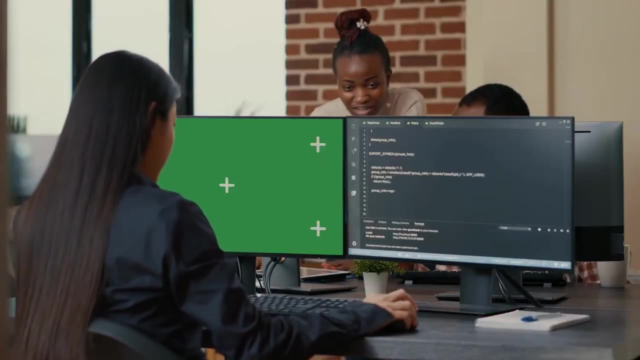 maintenance and troubleshooting. This trend will keep growing in the industry in the coming years. Also, companies will start to use AI to help customers help themselves. By following AI instructions, customers will be able to set up devices, fix problems and troubleshoot problems. 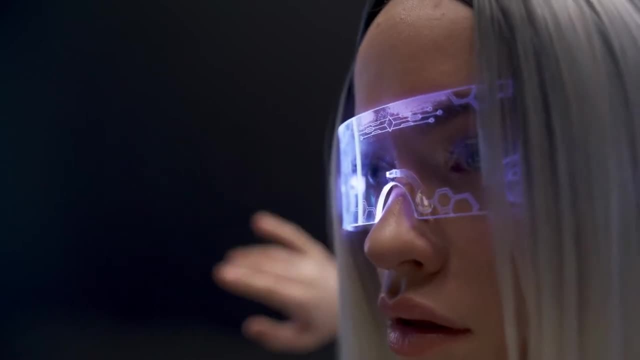 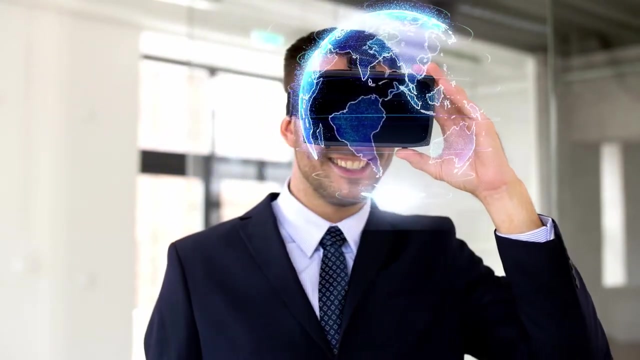 Use of connected devices. The growth of connected devices is another thing that will change in the telecom industry. The way the business world deals with the Internet of Things will have to change. The Internet of Things could connect trillions of new things in the future.